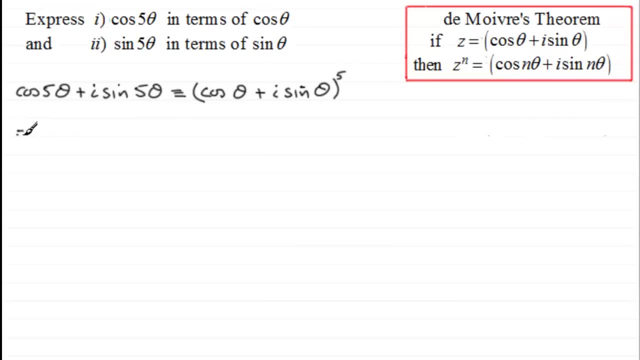 just move this to the side here. I'm going to rewrite this as being identical to c plus i s to the power 5.. C for cos theta and sine 5 theta. So what I'm going to do is just move this to the side here. I'm going to rewrite this as being identical to c plus i s to the power 5.. 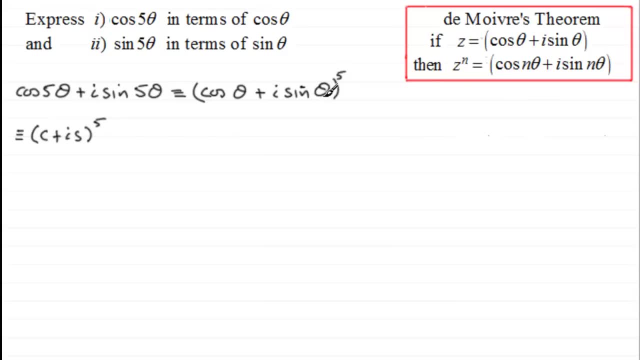 Thats equal to 1, 1, 1, 1, 1, and, and s for sine theta, and if i do expand this, then what we've got is that this is identical to, and. as many ways of expanding this, i'm going to use the binomial expansion using pascal's triangle. 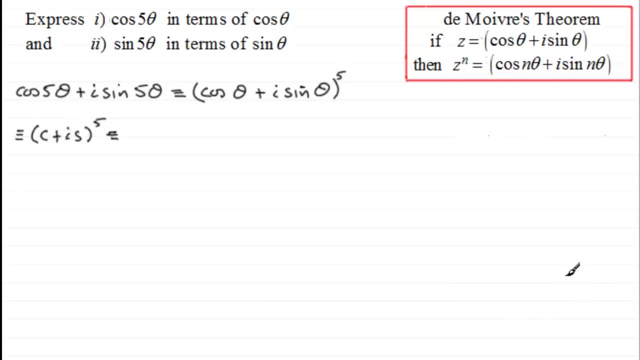 So I need to coefficients. So i'm going to write this down once and, starting with our one, we've got 1, 1, 2, 1, 1, 3, 3, 1, 1, 4, 6, 4, 1, and then for 5 it's going to be 1, 5, 10, 10, 5, 1.. 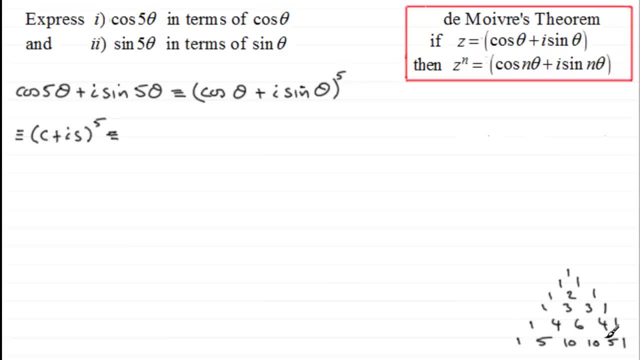 So I'm assuming you're familiar with Pascal's triangle, or you could use the combinations method of expanding this. So anyway, we end up with one lot of c to the power 5, so you've got c to the power 5 there. 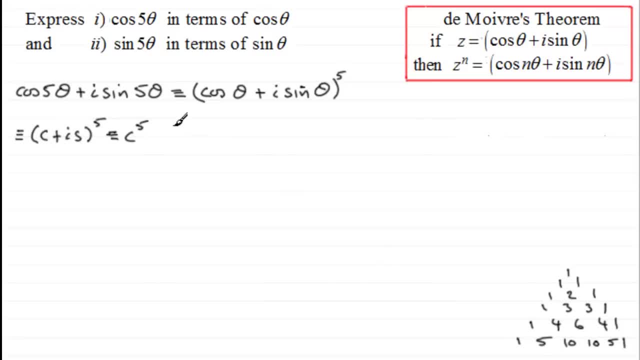 And then for the next coefficient, it's going to be plus 5, drop the power by c or by 1, and so that's c to the power 4, and introduce is to the power 1.. Next term is going to have a coefficient of 10.. 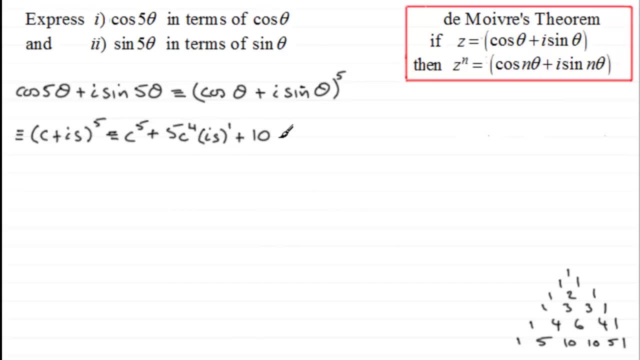 So it's going to be plus 10, drop the power on c by 1,, so it's c to the power 3, and increase the power on is by 1.. So it's now going to be up to 2.. 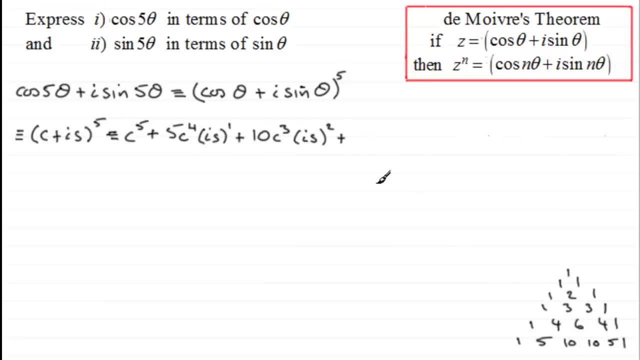 And we work our way down through these remaining terms. so we've got 10,. now we have c to the power, 2, is to the power 3.. Next term would be 5, and then c to the power 3.. 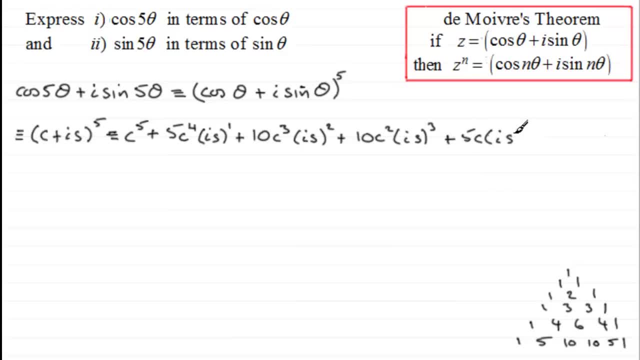 So that's c to the power 1,. I'll just leave it at c, and then is to the power 4.. And then final term would be one lot of c to the power 0,. that's just going to be 1, and then is to the power 5.. 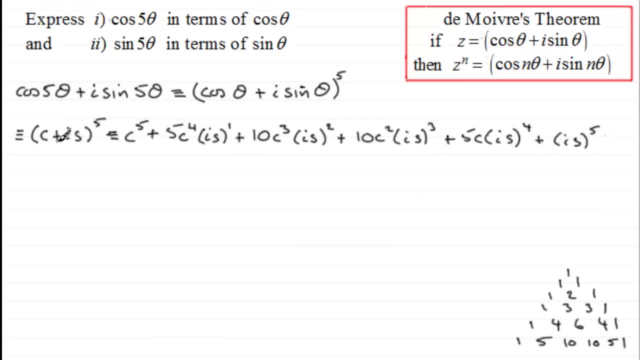 Okay, so there's your terms for the binomial expansion of that. Now, what I'm going to do next is group together all the real parts and the imaginary parts. Okay, so if we look at the real parts- and again I'm going to have to move over to here, because this is going to be quite long- 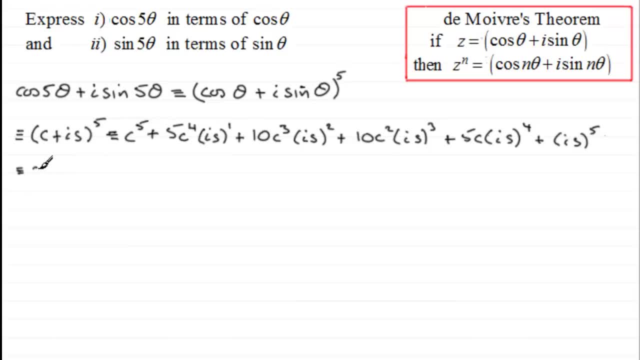 So it's identical to well, c to the 5 is real, and this term here is going to be i to the power. 1, that's going to be imaginary. This one here we're going to have i squared, that's real, because i squared is negative 1.. 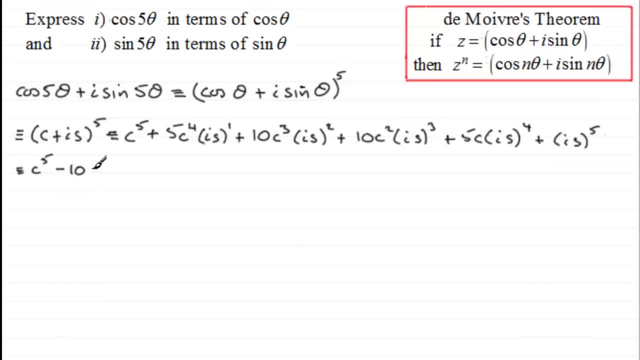 So we've got minus 10 c cubed and then s squared. Okay, this term here is going to be imaginary, with i cubed in it. This term will be real because it's going to be i to the 4.. i to the 4 is plus 1, so we've got plus 5 c, s to the 4.. 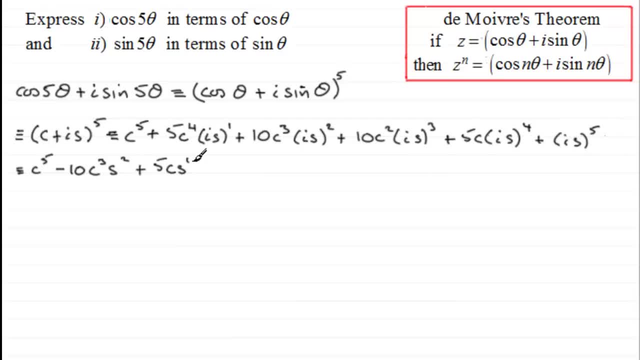 Plus 5 c s to the power 4.. Then we've got: the remaining terms are going to be imaginary. So I'm going to put i as a common factor out the front, And then what we've got is this term here which is imaginary. 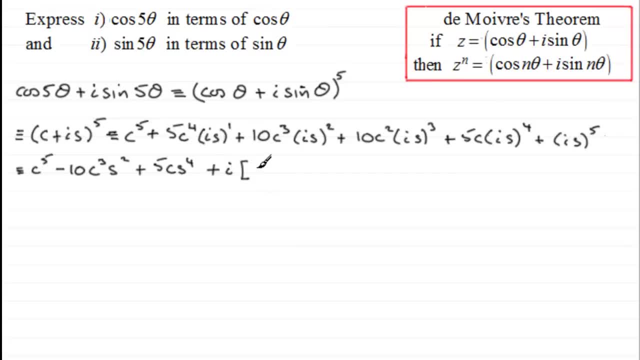 It's going to be 5 c to the power 4 s, So I put that in: 5 c to the power 4 s. This term we said was real, This term is imaginary. We've got i cubed. i cubed is going to be minus i. 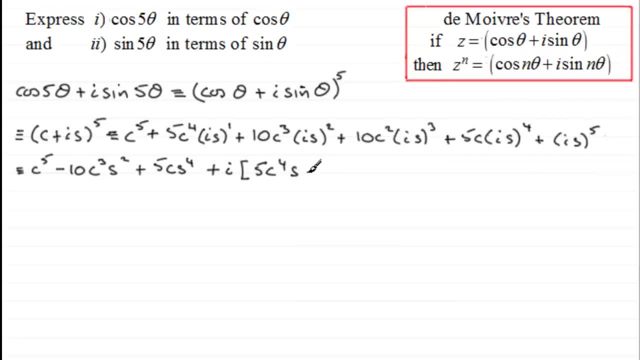 So we've got minus 10 c squared And then S cubed, And then we have this last term here: i to the power 5.. Well, i to the power 4 would be plus 1. Times it with another i. 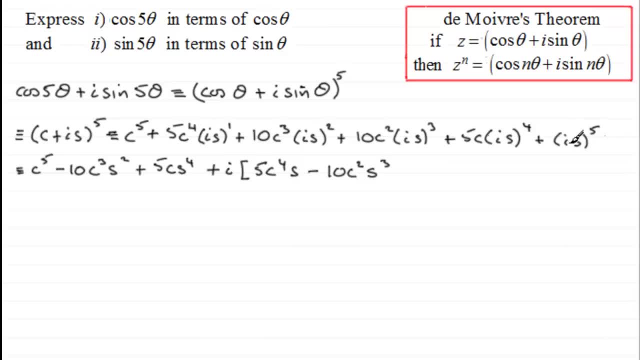 And you've just got i, So i to the power. 5 is just i, So you've got i s to the 5.. So plus s to the power 5.. Okay, Now, what we've got to do is express cos of i to the power 5.. 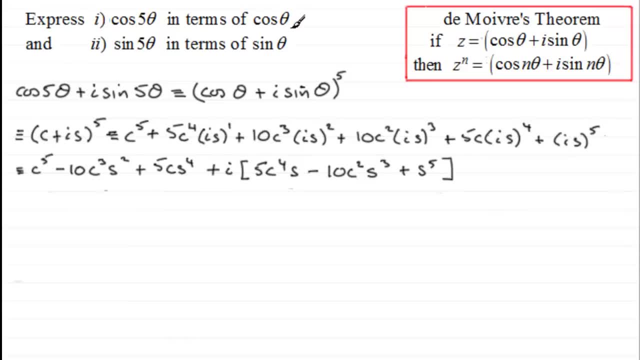 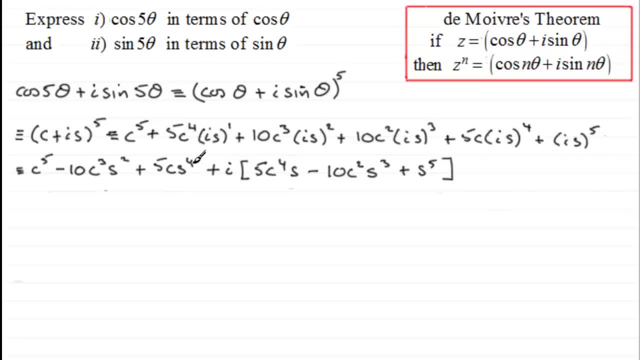 So we've got a few signs here, okay, which we need to change, And we can do this knowing the identity that sine squared theta is the same as 1 minus cos squared theta. So we've got for the first term here c to the power 5.. 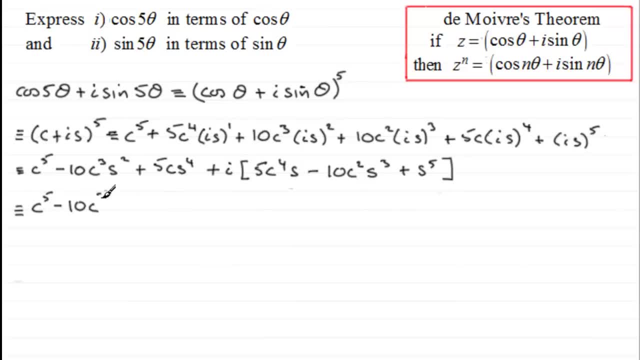 And then minus 10 c cubed. But in place of s squared, write that as 1.. 1 minus c squared. for this next term plus 5c, we've got s to the power 4. we can think of this as s. 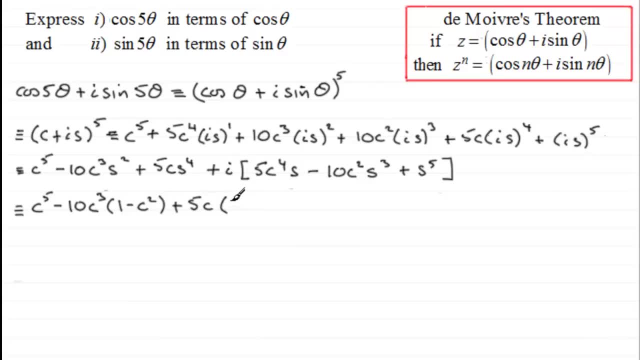 squared, all squared. so s squared was 1 minus c squared, and we just need to square that, okay, so that's the real part done. now we move on to the imaginary part. plus i multiplied by now for the imaginary part, sine 5 theta we've got to express in terms of sine theta. 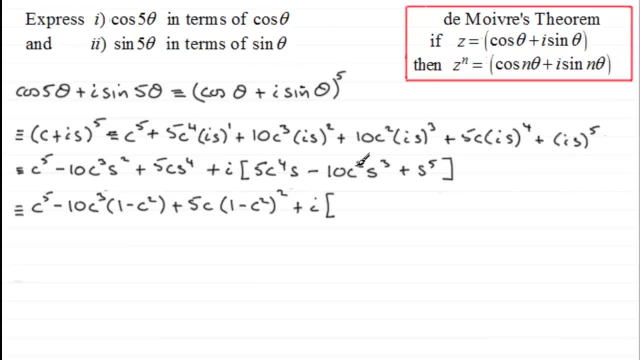 so we don't need these cosines here. okay, so we can pick up on the fact that c squared cos squared theta is 1 minus sine squared theta, and for c to the power 4, that's 1 minus cos squared theta all squared. so for this term here we've got 5s multiplied by. 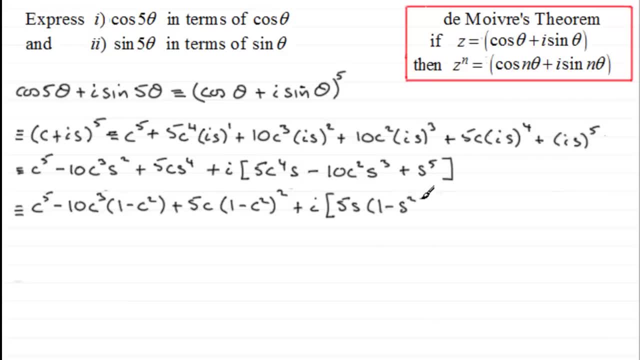 1 minus s squared, all squared, okay. and now for this next term, we've got minus 10s cubed multiplied by c squared. c squared is 1 minus s squared. and then we've got plus s to the 5- okay, and all we've got to do now is just expand all the brackets. 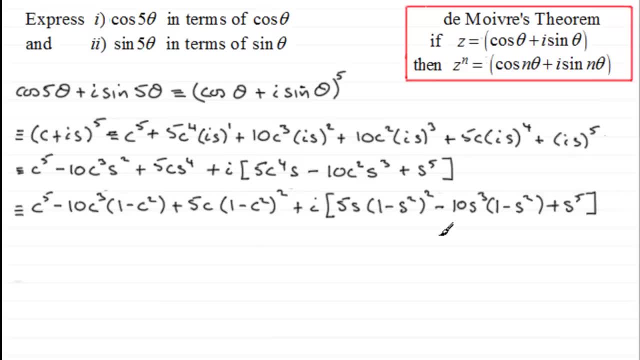 and then group up the terms and, to save time, you can check it. i've got it here, and if i now group up the real parts and the imaginary parts, i end up with the following: now that means that all i've got to do now is just compare the real parts and the imaginary.